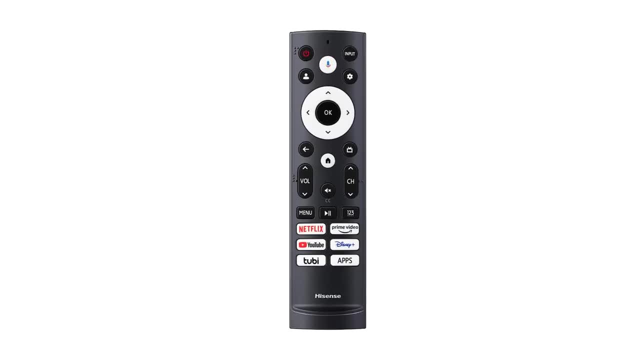 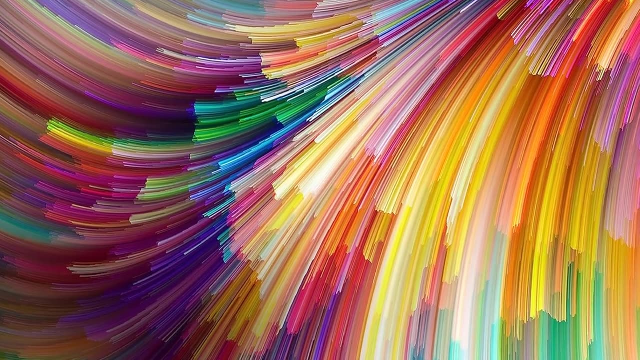 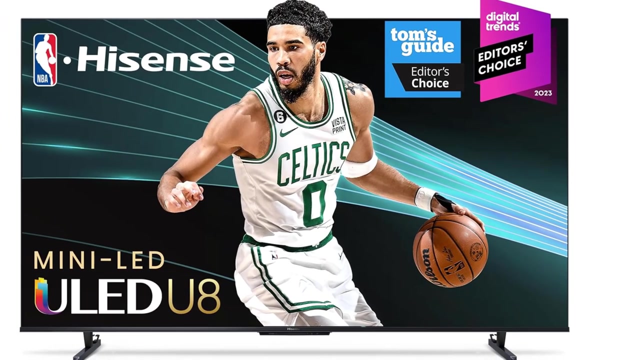 I set up my PlayStation 5 and tested the refresh rate with Persona 5, Dancing in Moonlight, a rhythm game. Colors are rich and eye-catching, while the high refresh rate eliminates motion blur and screen tearing that can ruin your watching or gameplay experience. 4K yield: Hisense's proprietary ULED technologies boost. 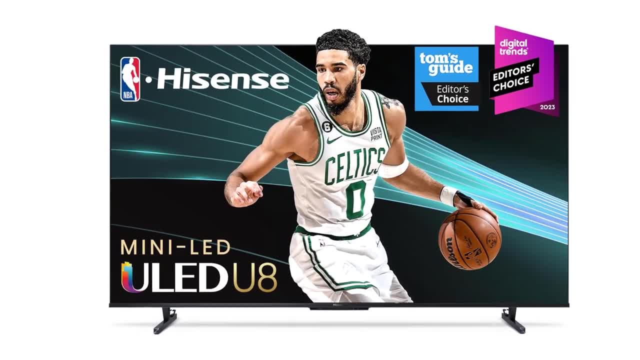 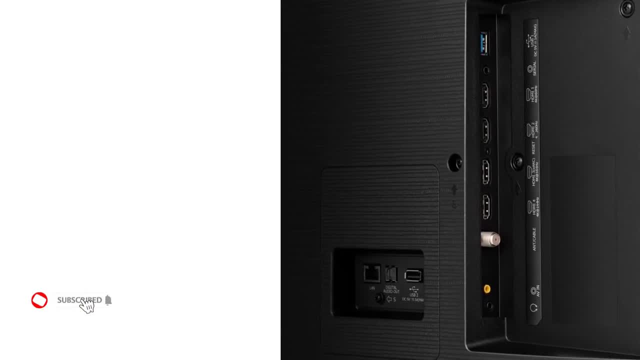 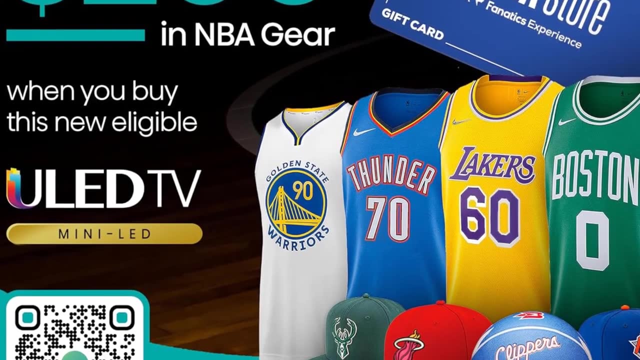 color contrast, brightness and motion. This suite of patented hardware and software technologies delivers an engaging and completely unique picture that can only be delivered by Hisense Mini-LED and full-array local dimming. Mini-LED is the latest breakthrough in backlighting technology By utilizing LEDs that are significantly smaller than traditional. 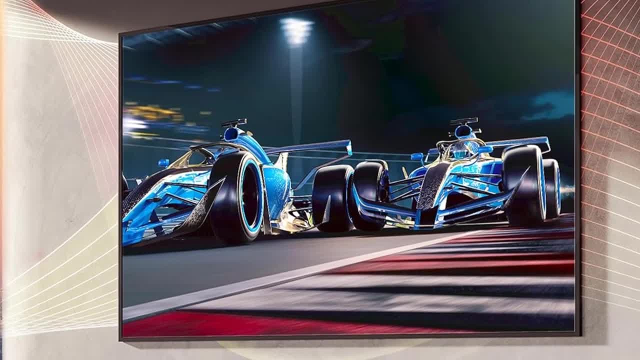 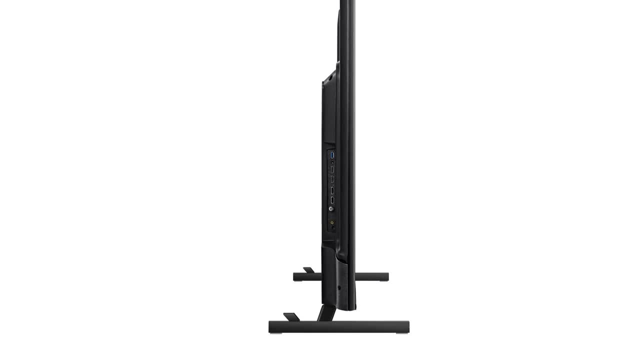 LEDs. we are able to use many more LEDs to create a bright image that distributes the light more. evilly for a uniform image across the screen. KLED, Quantum, DOT. Wide Color Gamut- QuantumqLED produces purer, richer, more brilliant and accurate color than a regular LED TV, Creating over a billion color combinations. 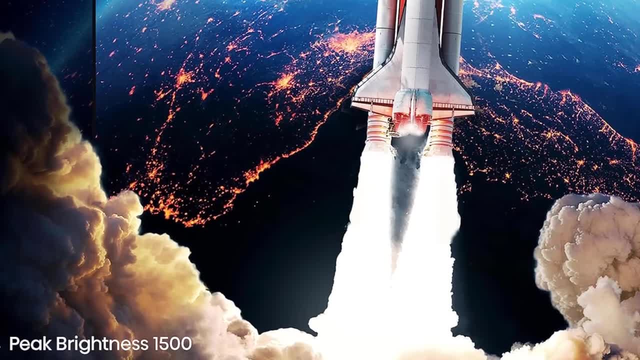 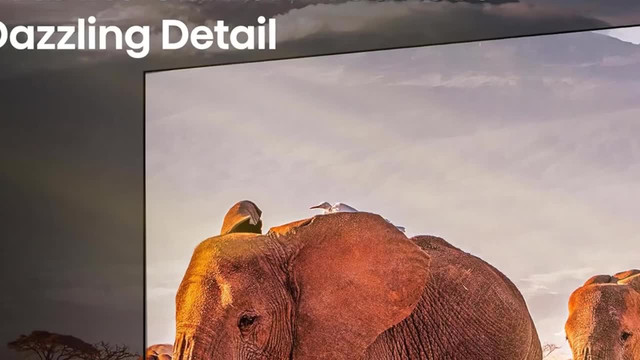 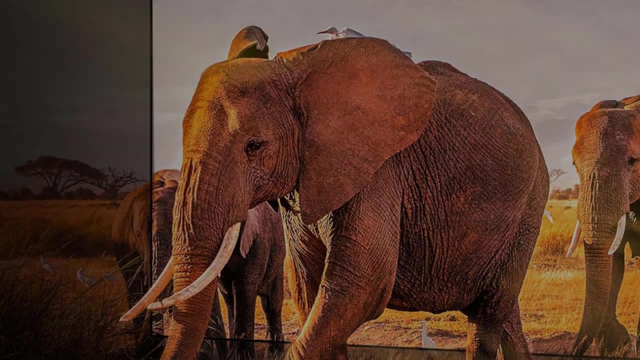 that bring vibrant images to life in a way non-qLED TVs can't, For 80 smooth motion and 144Hz native refresh rate. smooth motion removes the digital noise that can affect moving objects. The TV's native 144Hz refresh rate is the foundation for its 480 motion rate. 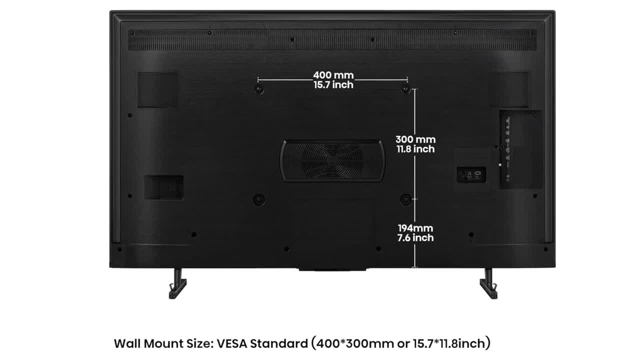 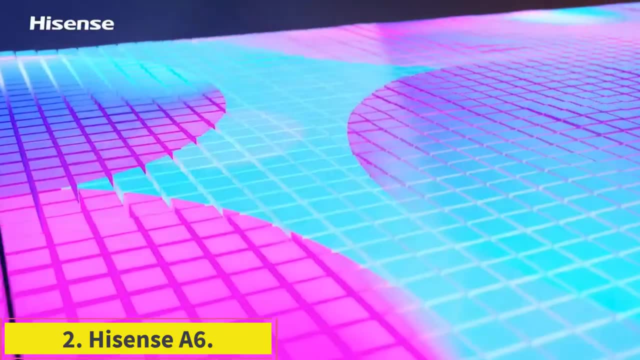 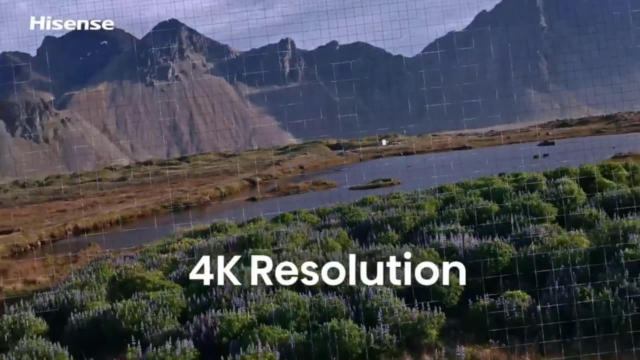 These technologies work in concert to make fast action scenes to ensure moving objects have minimal time. Number 2. Hisense A6.. If you're working with a smaller budget or want a new TV with a smaller screen, the 43-inch Hisense A6 is a great option. It retails under $300, which means even very 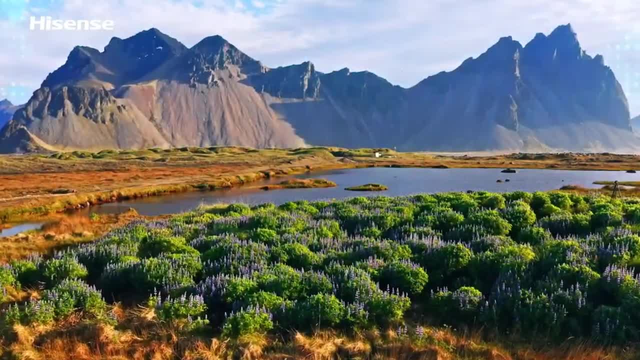 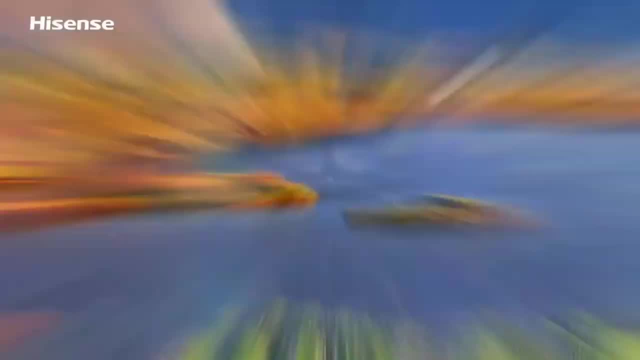 meager budgets can find room for it And you won't have to sacrifice features you've come to expect as standard for home entertainment. you'll still get great 4K resolution as well as Dolby Vision support for enhanced picture quality. It also supports DTS, which is a great feature for home entertainment. 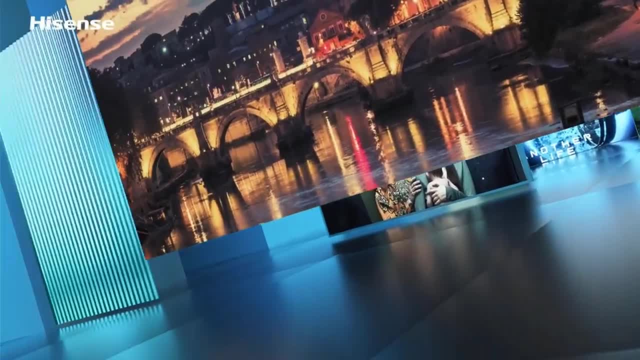 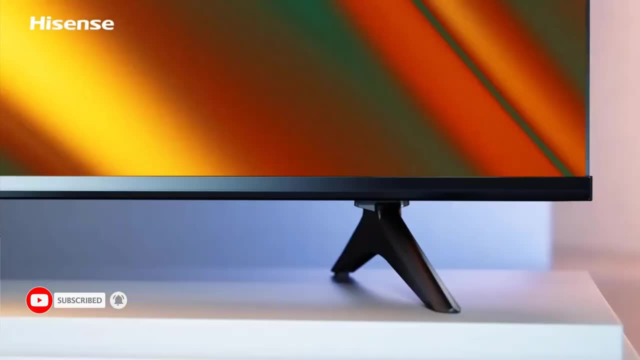 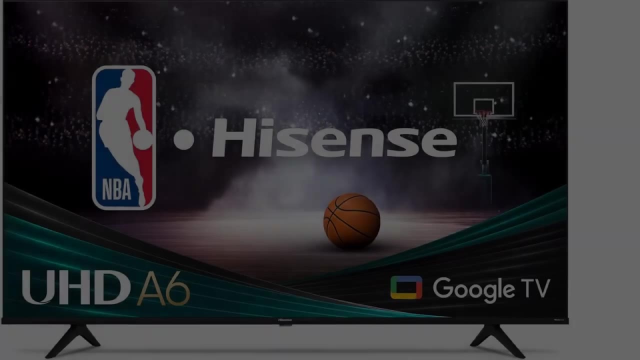 It also supports DTS Virtual X for a better listening experience while watching movies and shows or streaming music. It has Chromecast built-in for sharing media from your Android devices, while the voice remote supports both Alexa and Hey, Google virtual assistants. 4K ultra-high definition, more pixels on the screen- produces a more clear and succinct 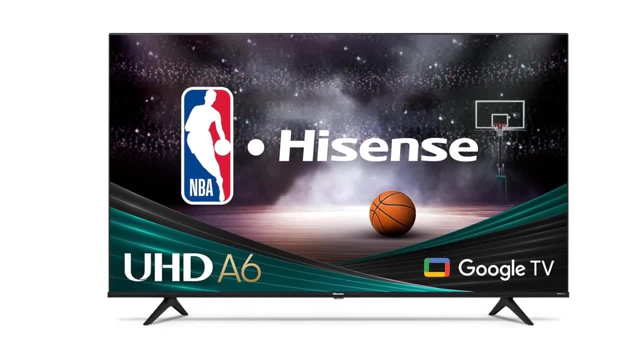 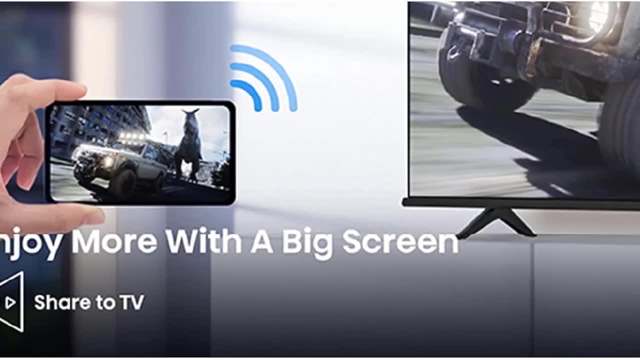 picture-making content look more realistic and true to life. Combined with Hisense's AI UHD upscaler, non-4K content will get enhanced to near 4K quality. Google TV- The entertainment you love. With a little help from Google. 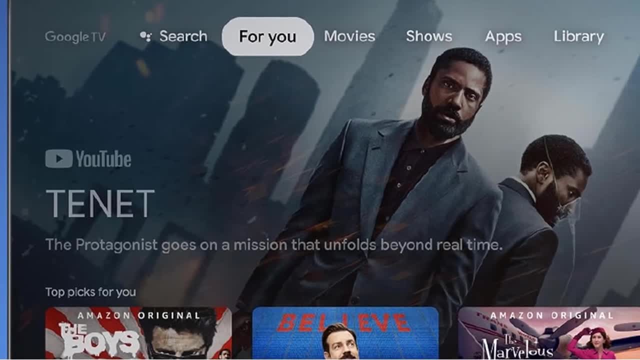 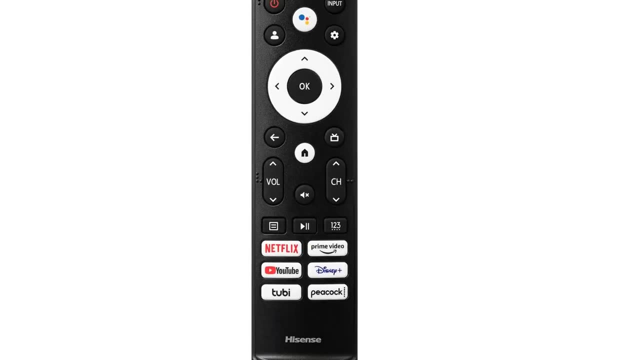 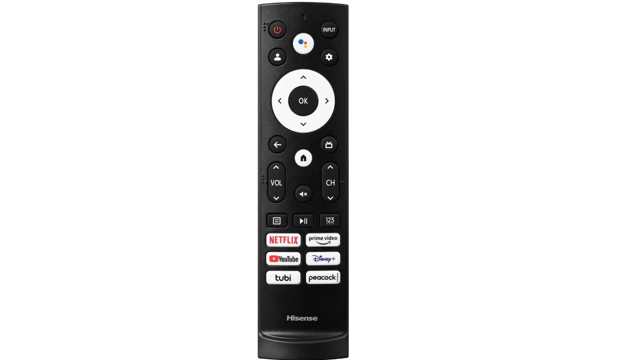 Google TV brings together movies, shows, live TV and more from across your apps and subscriptions and organizes them just for you. Dolby Vision, HDR and HDR10, innovative visual technology. Dolby Vision brings the characters to life with darker darks, brighter brights and a remarkable color range you can't get anywhere else. 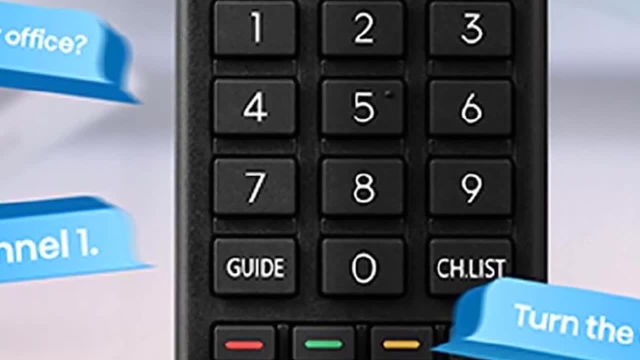 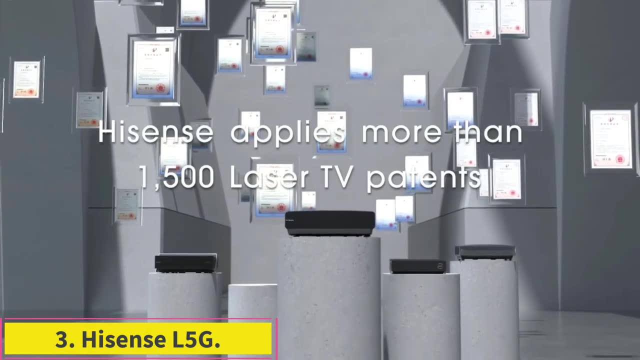 HDR10 is an HDR format that delivers HDR content via compatible over-the-air signals. Number 3. Hisense L5G. If you're looking for a high-end TV for your home theater, you should check out the Hisense L5G. 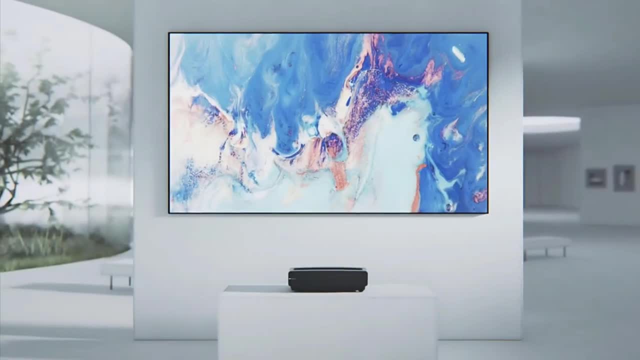 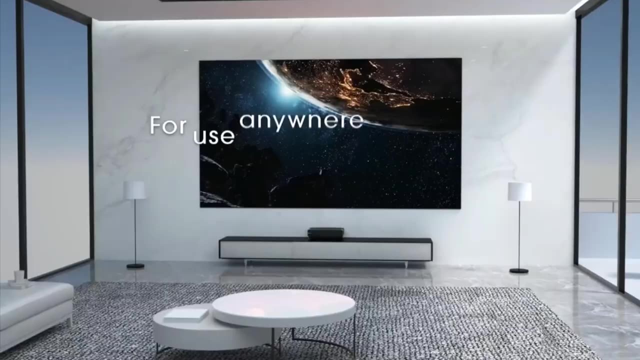 It's a short-throw laser projector, which means you won't need a giant room to set up your TV, but you will need a large wall for the up to 120-inch screen it comes with. The screen is designed to reject ambient light for a more clear image. 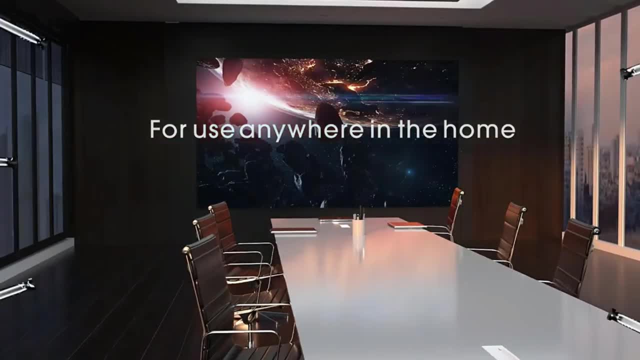 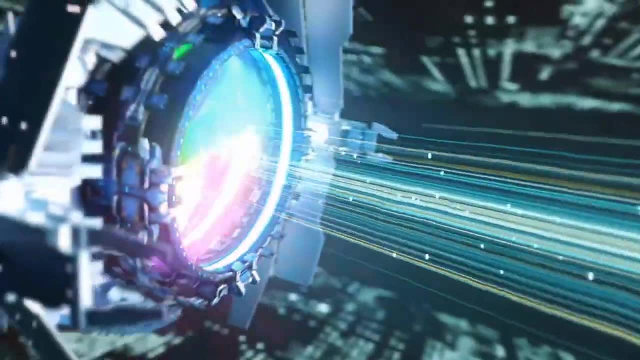 The projection unit laser has a 25,000-hour life expectancy, which means that you can watch the barcodes movie-slash-Oppenheimer double feature on loop over 5,100 times before it stops working. The laser also can produce up to 2,700 lumens of brightness. 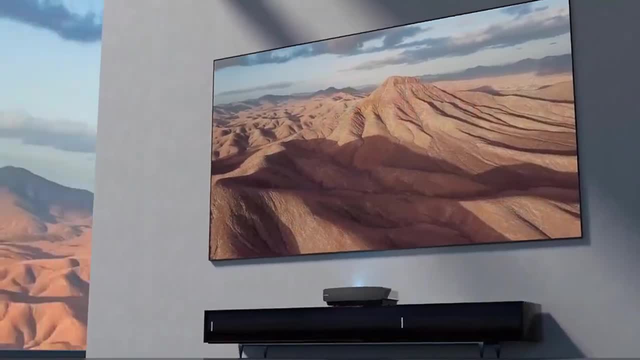 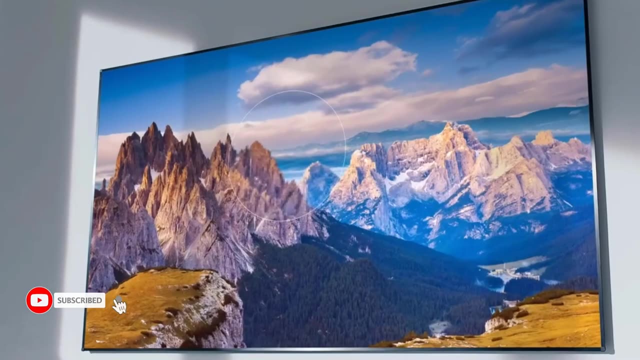 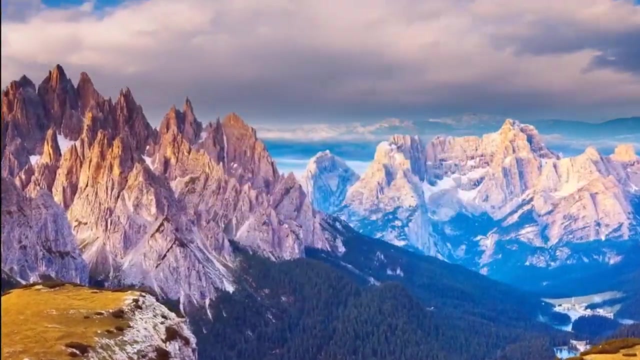 so you won't have to wait until after dark to fully appreciate the L5G Big screen entertainment in a convenient package. No need for ceiling mounts or in-wall cable runs. simply place the L5G on a TV stand just 14 inches from the wall and get a massive 120-inch projection. that's 4x more screen than a 55-inch TV. 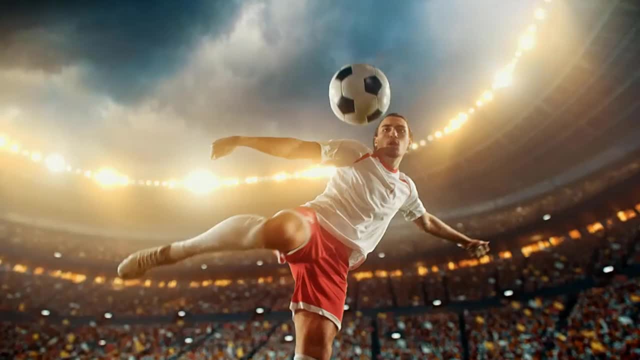 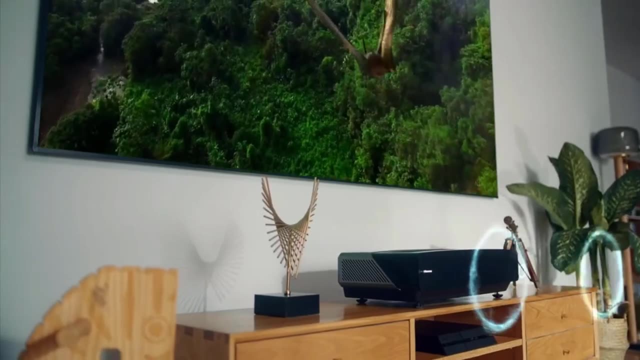 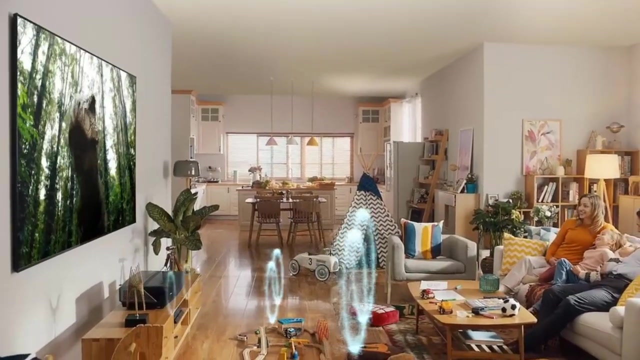 The L5G comes with a perfectly paired ambient light rejecting ALR screen to remove the guesswork from a UST projector setup. The UST ALR screen gives you a killer picture under any lighting condition without having to kill the lights. With built-in 30W Dolby Atmos sound, the L5G delivers cinematic sound that. 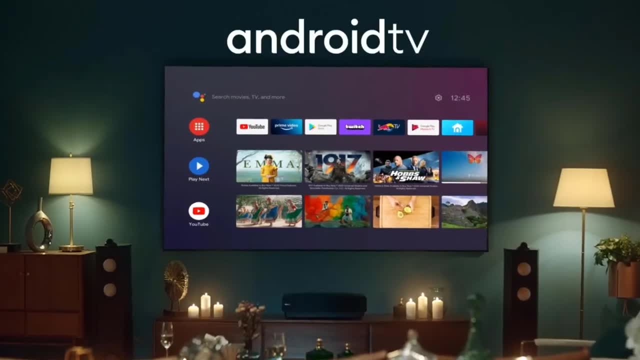 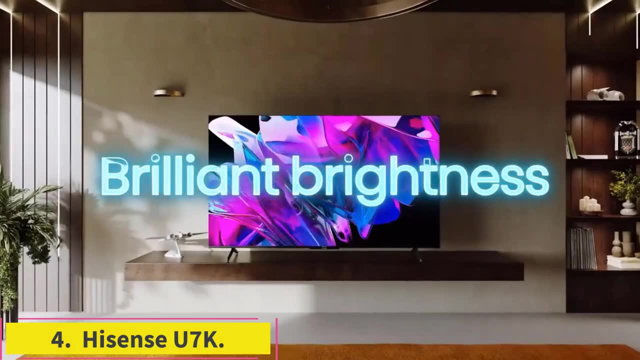 seemingly flows all around you. For the true audiophiles, the L5G Z Arc support means you get full signal pass-through to your surround sound system. 4. Hisense U7K. The Hisense U7K is a great choice for a big-screen TV.